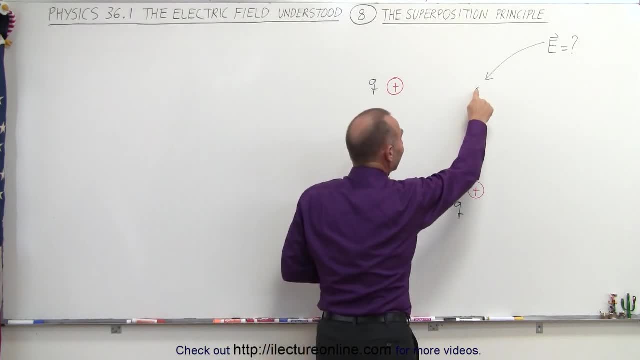 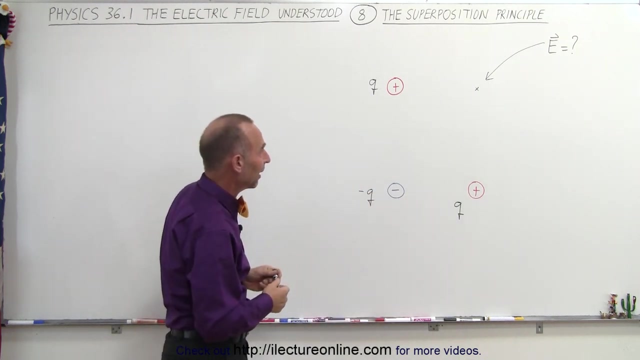 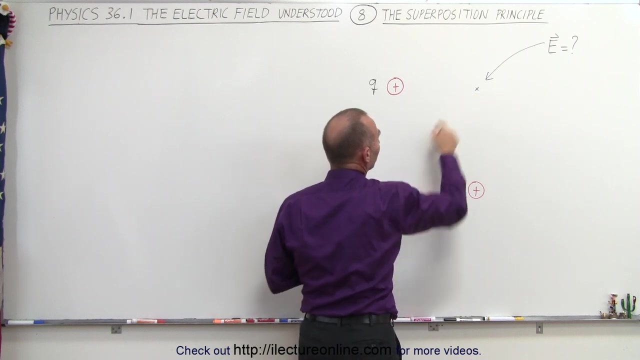 states that the electric field at this location is simply a vector sum of the electric field created by this charge, by this charge and by this charge all added together. So let's go ahead and illustrate that and then later on we'll see some examples of that. So the electric field created by this charge right here of course emanates in all directions, but relative to this point right here, we can see that there's going to be an electric field in this direction. 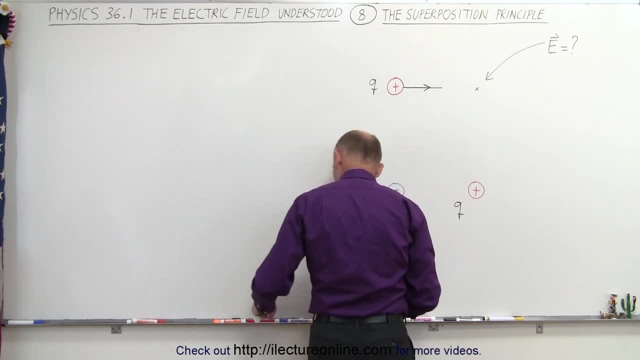 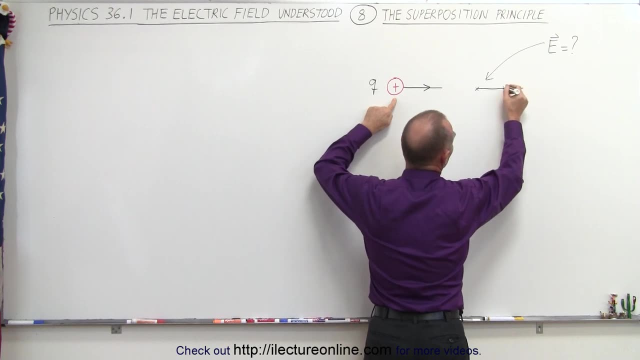 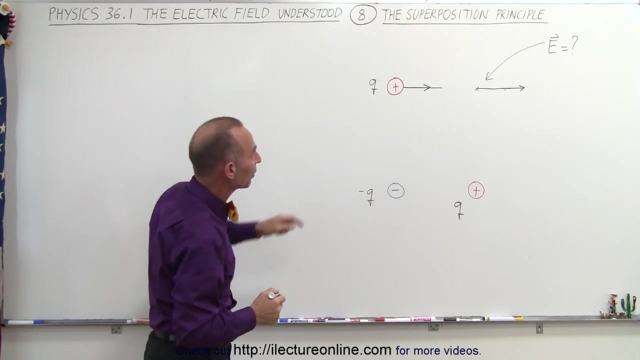 Like so: So at this location, we can indicate that there's an electric field from this source, from this source at this location, in this direction. So let's go ahead and draw it like this. And actually what I'm going to do is I'm going to just draw a vector like that, the vector arrow that indicates that the length of the vector represents the magnitude of the electric field caused by this charge right here. So I'm going to call this Q1.. 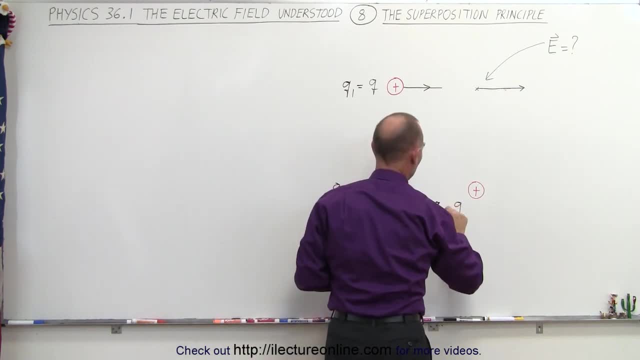 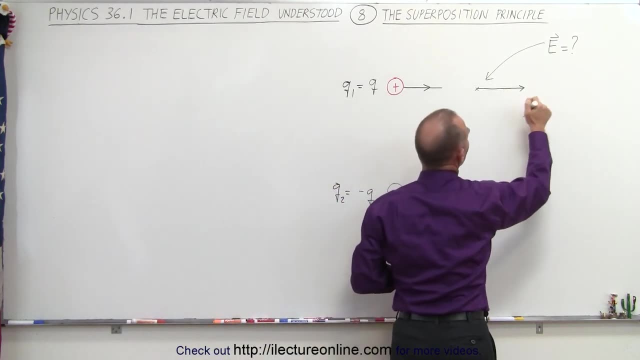 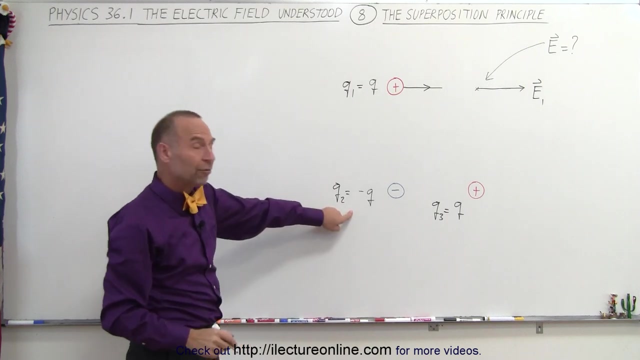 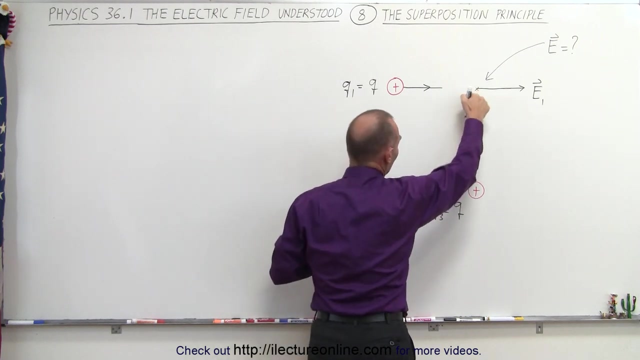 I'm going to call this Q2.. And I'm going to call this Q3 because it's easier to keep tabs of what is what when we draw that. So this here would be the electric field as produced by the first charge, Q1.. Now we can do the same for Q2, except here we have a negative charge, which means electric field emanates towards the charge. So from this direction to here we can see that electric field would be caused to be in this direction. 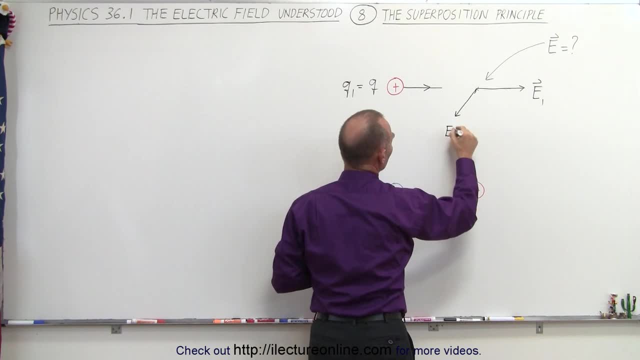 By this charge, and so we'll call this E2.. And then, finally, the electric field caused by this charge, since it's a positive charge, will be away from the charge, And so when we get over here, the electric field will be in this direction, and we'll call that field E3.. 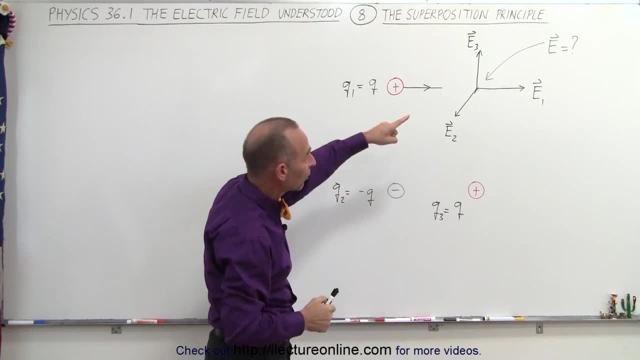 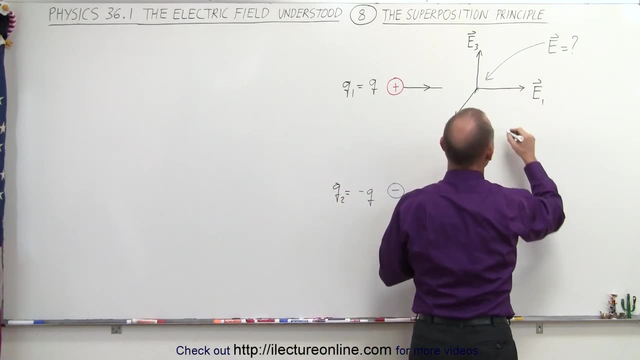 Now to find the net electric field at that location, we would simply add those three vectors together: E1 plus E2 plus E3.. So we can say that the electric field is in this direction And the electric field at that location is simply the vector sum of E1 plus E2 plus E3..